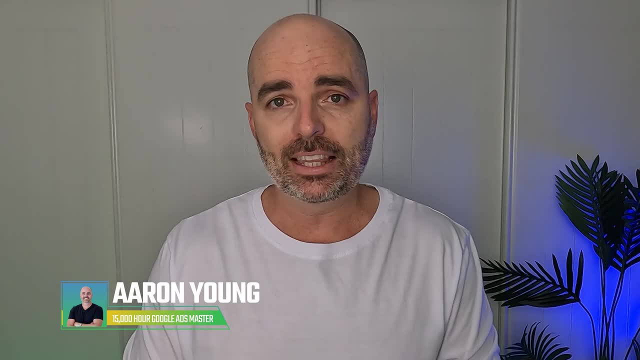 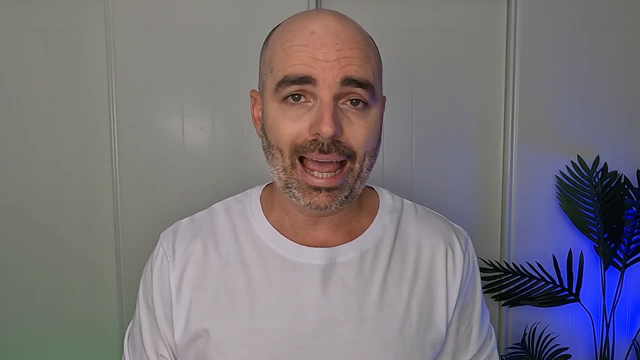 my name is Aaron Young, I'm from Define Digital Academy and I'm your 15,000 hour Google Ads master, And the very first strategy that you need to undertake in order for success with Google Ads- if you've got a small budget- is that you need to make sure that you've set your budget at a 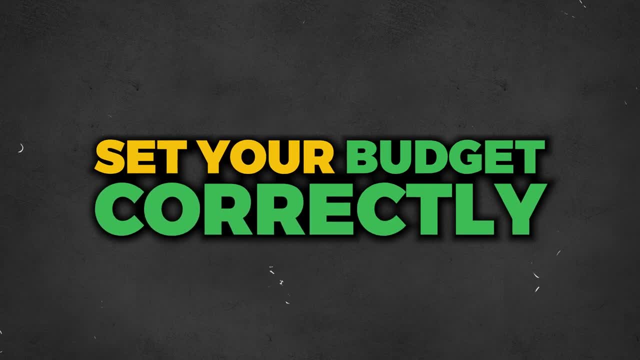 high enough level that you're going to be getting enough data to be able to do the job that you're going to be doing. So you need to make sure that you're getting the right data and volume through your Google Ads campaign Now. the reason for why this is so important is because you need to make 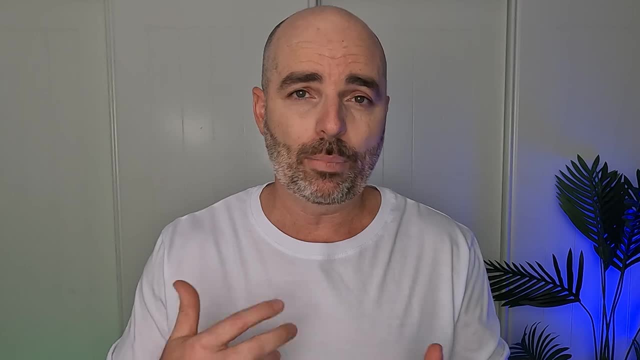 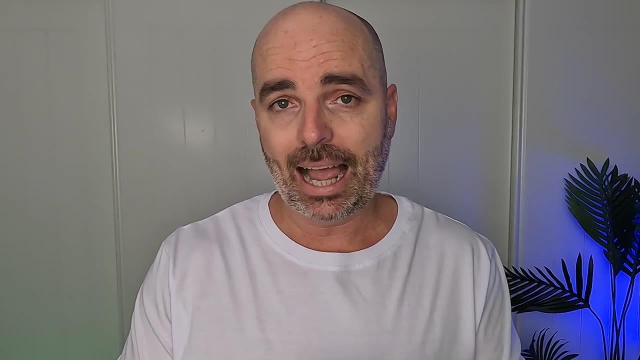 sure that you're getting a baseline level of data and volume, And by that I mean a baseline level of impressions and clicks. And this is important because if you're not getting enough data going through, you don't have enough data to be able to view your data and also then make some extra. 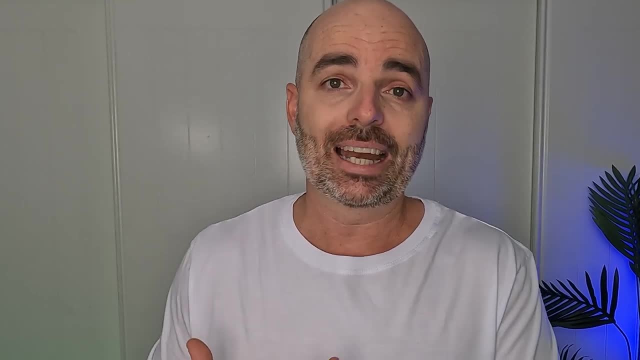 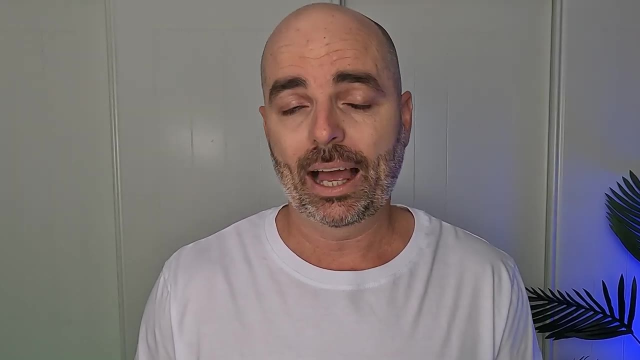 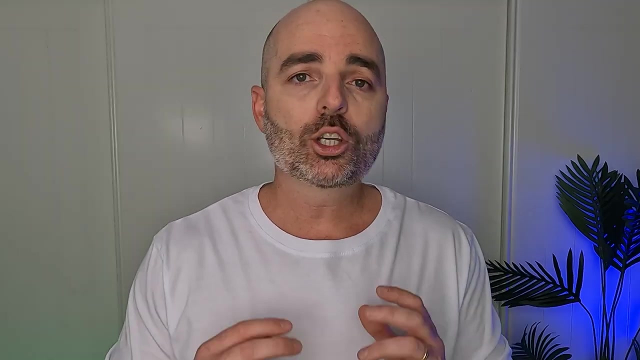 optimizations, But also as well. Google is not able to get enough data to be able to run its baseline split and optimizations so that it can automatically start filtering out the best traffic for your campaigns. And I know you're asking right now: how much data do you need? Well, as a good rule of 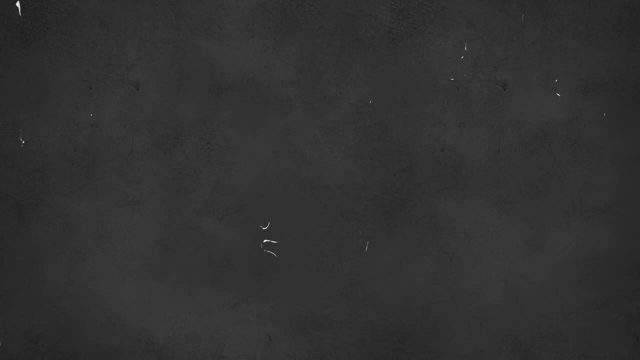 thumb. these are the metrics that you should be achieving with the absolute minimum goal that you need to be getting at least 10 clicks a day. Now if we were to roll that out, if you're running a search campaign with a baseline click through ratio of 5%, so you're getting five clicks out of 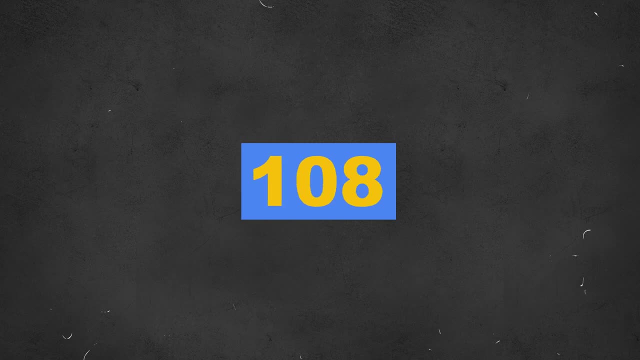 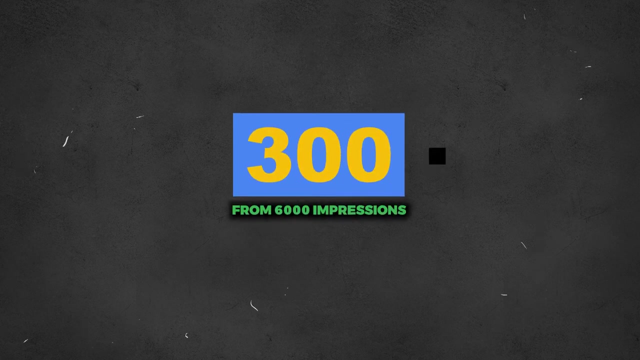 every 100 impressions. that means that you need to be getting 200 impressions a day. So when you take it out to a month, you'd be looking at getting 300 clicks a month from 6000 impressions. Now if you're running performance max, that click through ratio comes down to about 1% as an initial. 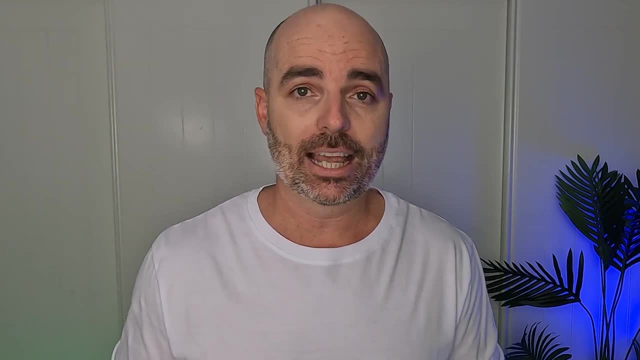 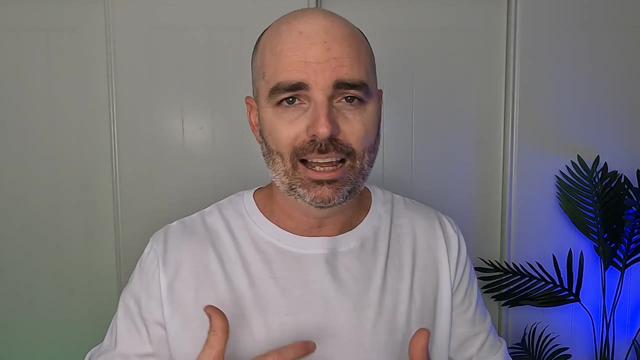 benchmark. So for those 300 clicks, you'd be needing to get 10,000 impressions a month And that is going to give you enough data, as I said, so that you're not in this endless learning loop where you're just not seeing enough data Because 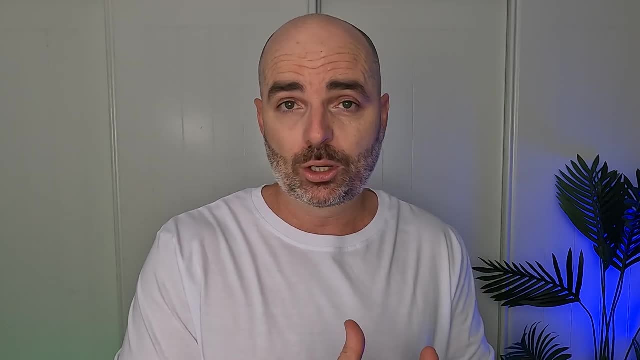 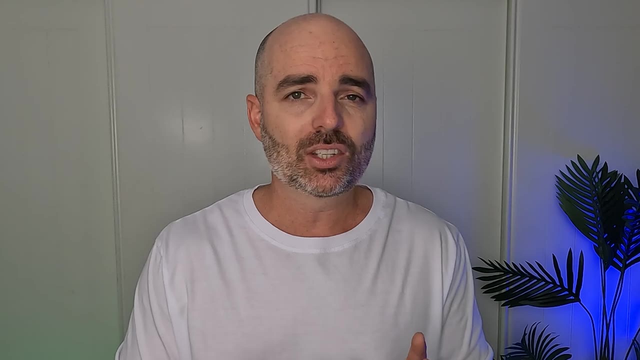 if you're only getting one or two clicks a day, you don't have enough data because by the end of the day that would only give you sort of 50 or 60 clicks And Google wouldn't have enough impressions, because a good benchmark is that Google needs for search campaigns at least 5000 impressions in a 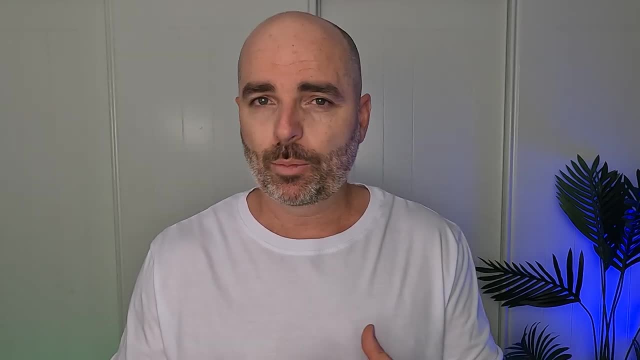 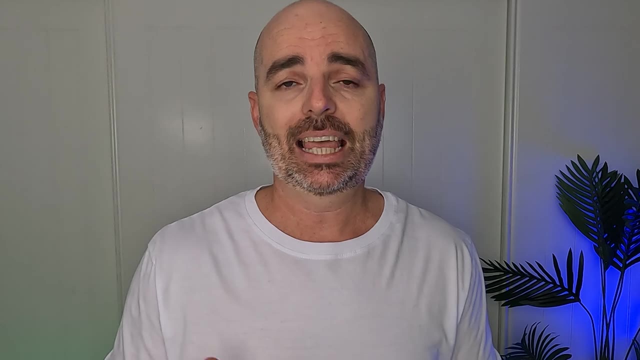 30 day period. Now there is some data to say that that is now down to about 2000.. But I still prefer to err on the side of caution and give Google more data, So that's why I'm still recommending to hit that. 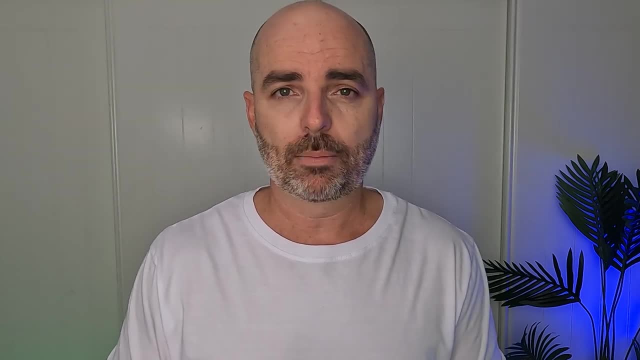 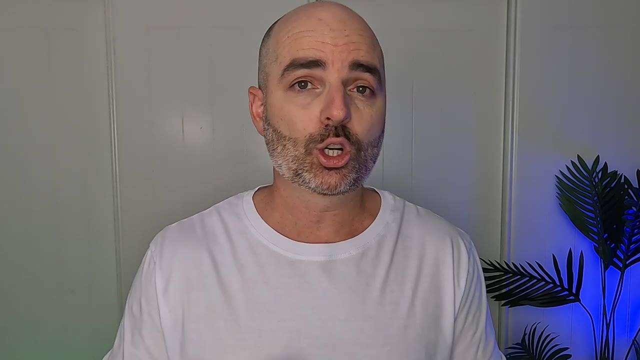 baseline of 5000 impressions in 30 days for a search campaign. So if you roll that all down, a simple way of setting your daily budget would be to find your cost per click, So the average cost per click for the initial product or keyword that you're going to be focusing, and then times that by 10.. So let me show you what I 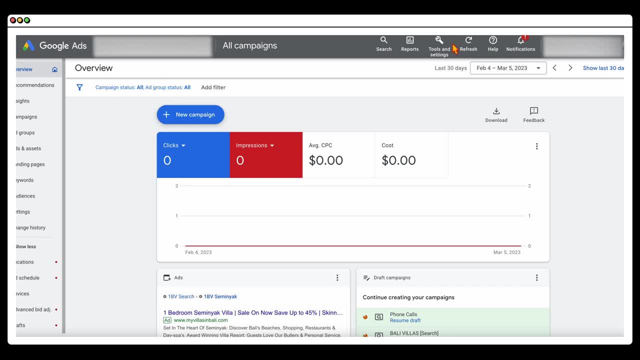 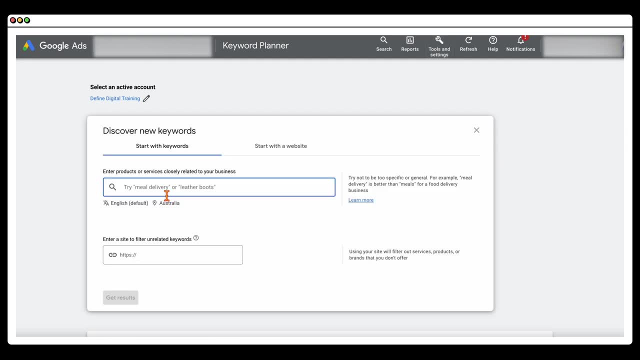 mean So to find this when you're in Google ads, if you go into your tools and settings, then go over to your keyword planner and then we want to go into discover new keywords. let's just say that you're wanting to do a campaign for iPhone 12.. 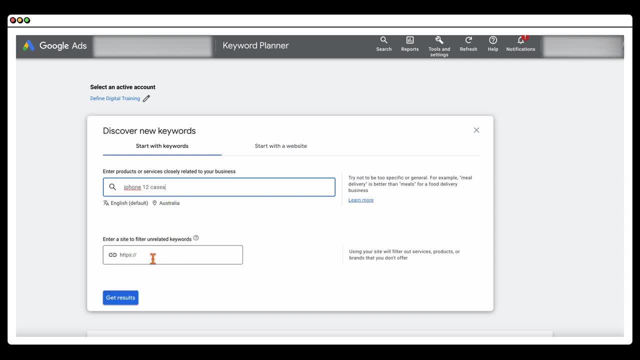 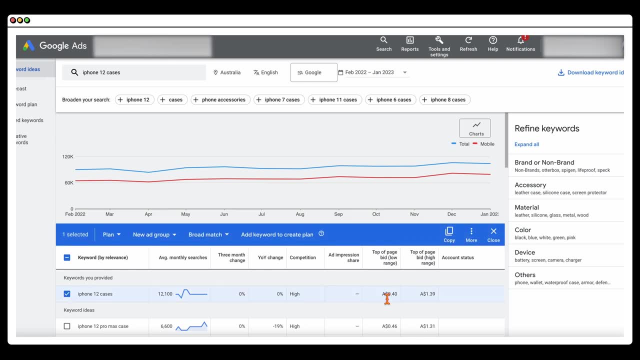 cases. So we type that in here, you can also add in your URL here. then you click Get results. So from here we can see there's a keyword for iPhone 12 cases And we can see here that the top of page bid for the low range- So those positions three and four- is 40 cents where the top of the 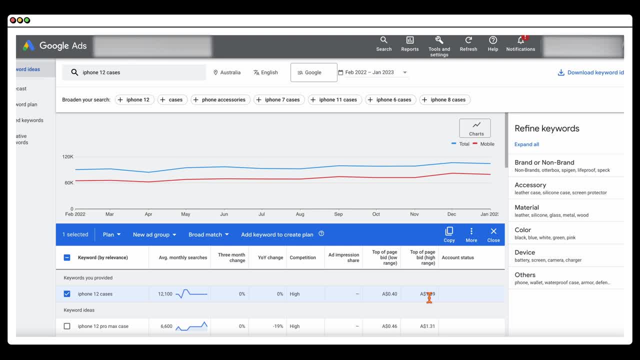 page bid for high range is $1.40.. So you'd be looking at there. I'd be wanting to take this number here and timesing it by 10.. So you'd be looking at that. you'd want a daily budget of $14.. As a minimum. 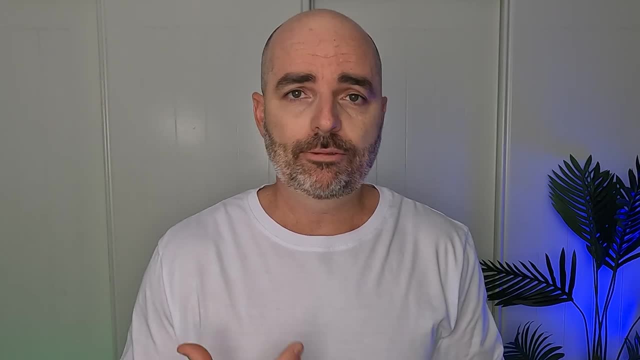 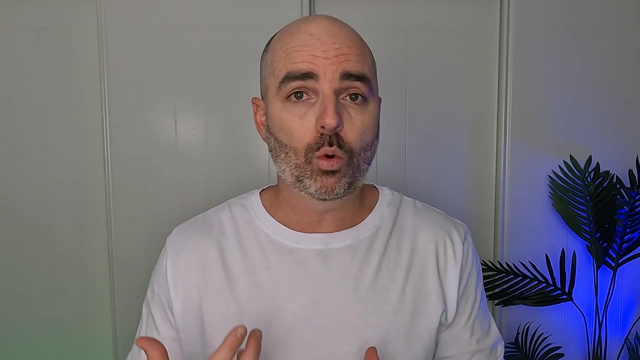 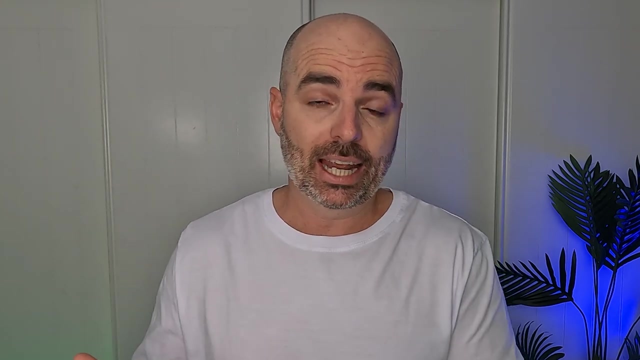 in order to get those 10. clicks. So that's the real simple process and formula you can use to get your initial starting budget is: go through and do that keyword research, find one keyword that you're wanting to focus on- so an individual product or an individual search term- and then times that average CPC by 10.. So in the example I showed you, the average CPC was $1.39.. And we times that by 10.. And that's why we'd be recommending a daily starting budget of $14.. Now, one thing I do want to stress with that is to also make sure that you're reviewing the data correctly and also making those correct. 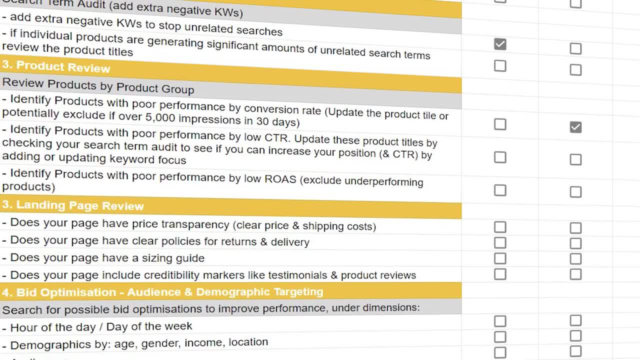 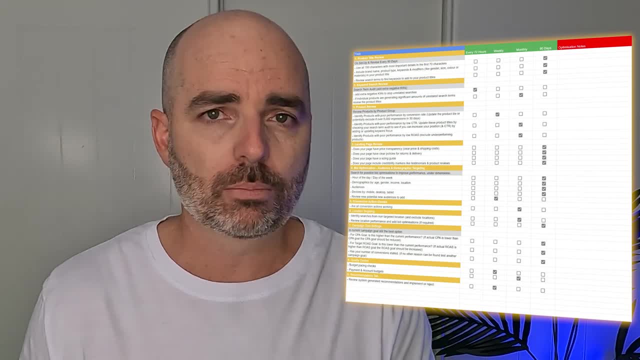 optimization decisions. I want to give you free access to my Google Ads optimization checklist, And this is a checklist which lets you know exactly what optimizations you need to be completing and how often you need to complete them, So whether they need to be done every 72. 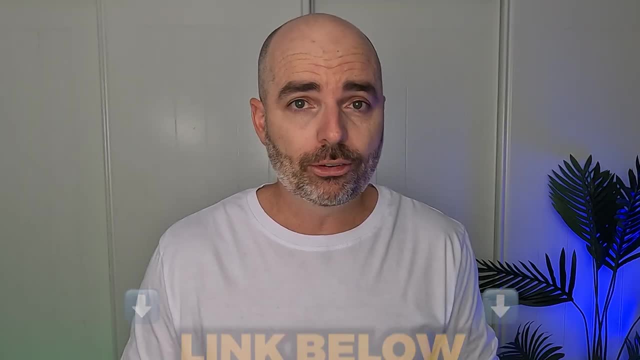 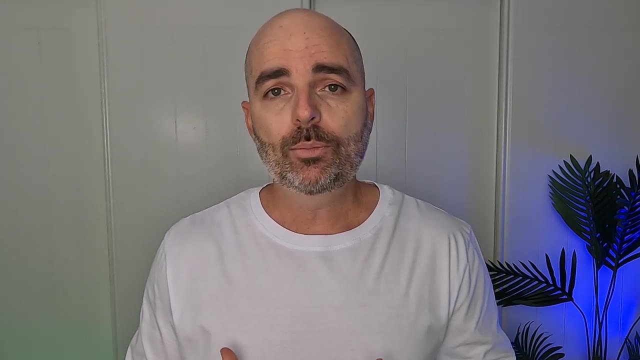 hours every week, every month or every 90 days, And if you want to get your free copy right now, all you need to do is to follow that link in description below. And now that brings us to the second strategy that you need to be using. 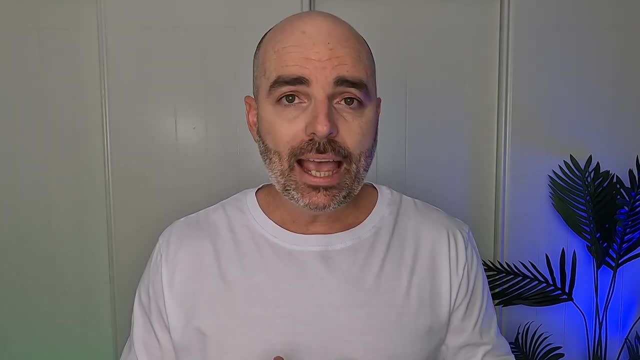 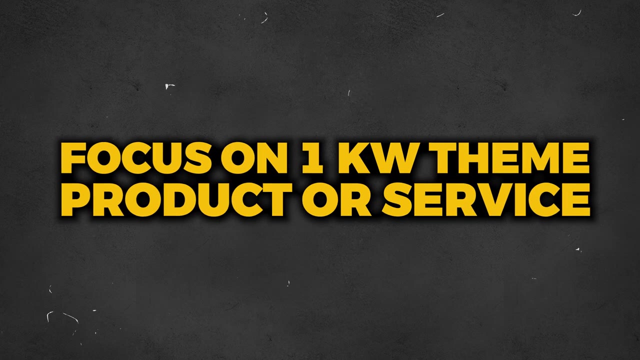 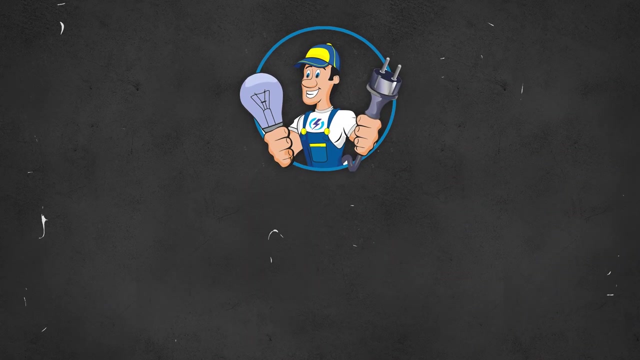 If you only have a small budget for Google Ads- and that is- is that when you start, you only want to focus on one individual keyword, theme, one product or one service. So if you have three different services that you're targeting- say, for example, you are an electrician and you- 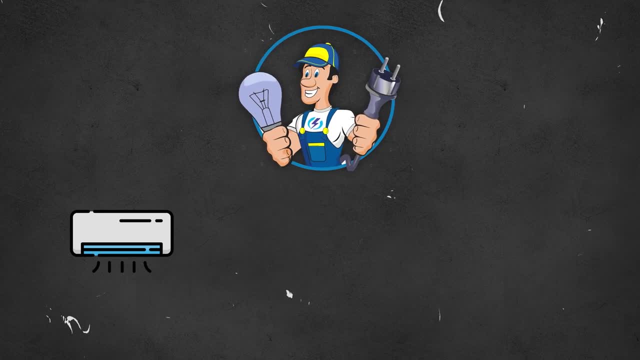 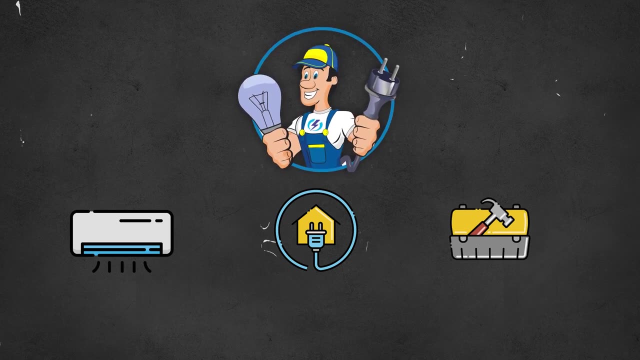 want to target air conditioning installations, you also want to target general electrical maintenance, or you also want to target little handyman jobs. I would just be choosing one of those things say, for example, air conditioning And for general maintenance, I would just be. 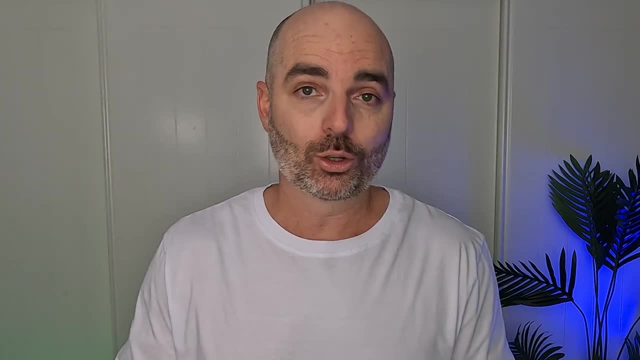 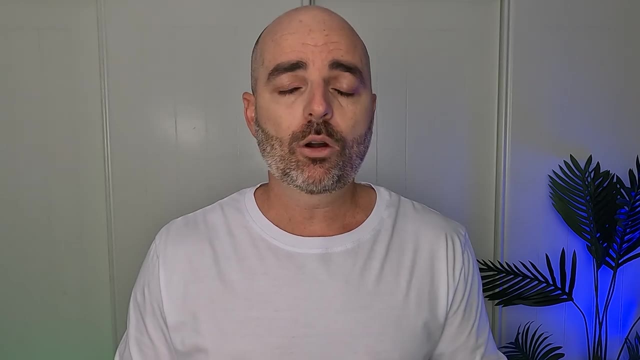 getting about those other services initially. when it comes to marketing on Google, And to also help you choose which service or product that you should be focusing on first, I would also say that you're better off to focus on your most popular or your highest selling product. And the reason for. 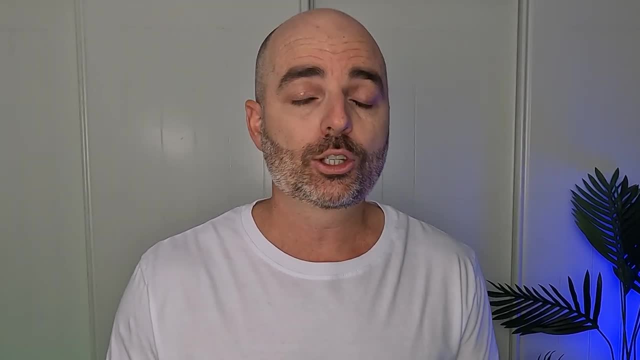 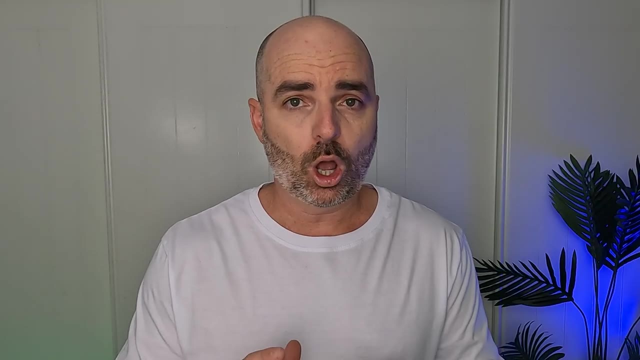 that. so the reason why you only focus on one product, while also focusing on your most popular product, is that it's increasing your chances for success so much more. So, firstly, the reason for why you'd want to only focus on one product or service or keyword theme is you've already got a. 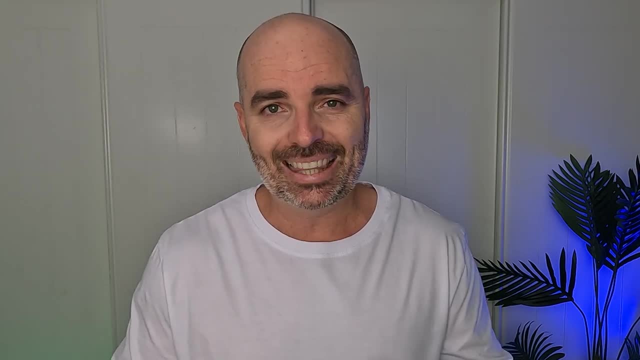 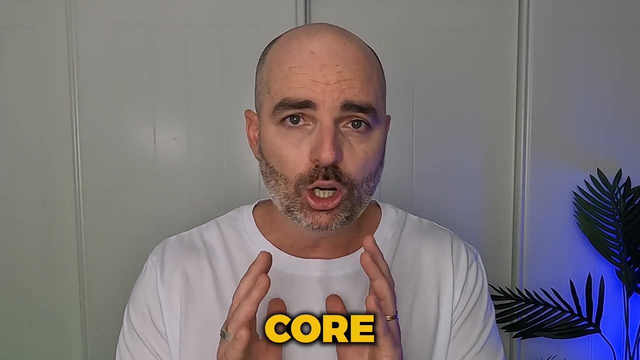 small budget, So you don't want to be spreading that budget any thinner by trying to target multiple products or multiple keywords or multiple services. just focus on one core product that you know will sell well And then, on top of that, the reason for you want to focus on one of your most 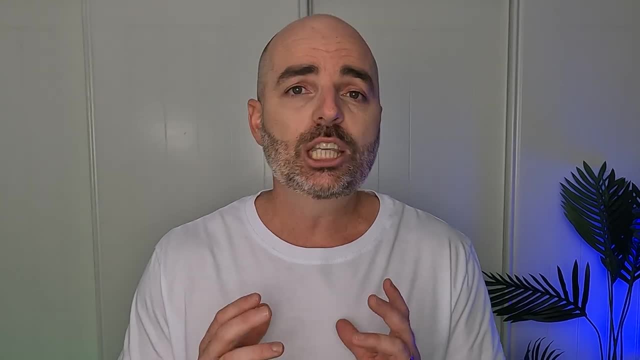 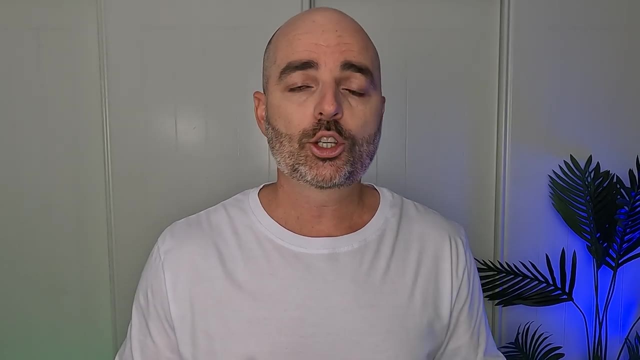 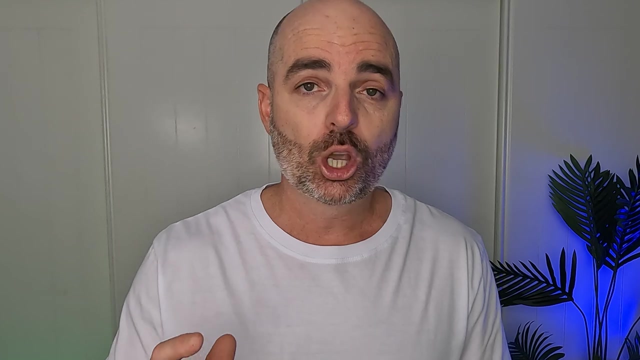 popular or your best selling services or products is because you know that they convert. you do know that people like your products or those particular services. So what you're wanting to doing is you're wanting to increase your, the amount of sales or revenue that that popular service already gets, so that you can then reinvest. 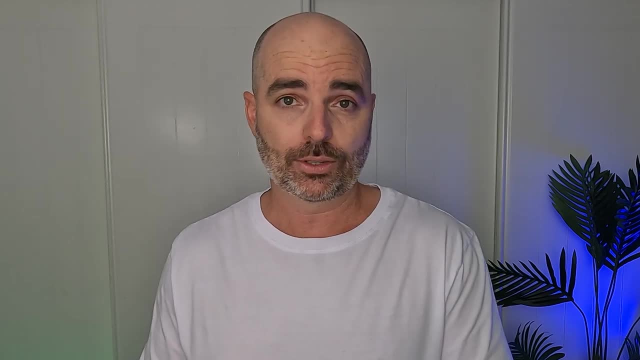 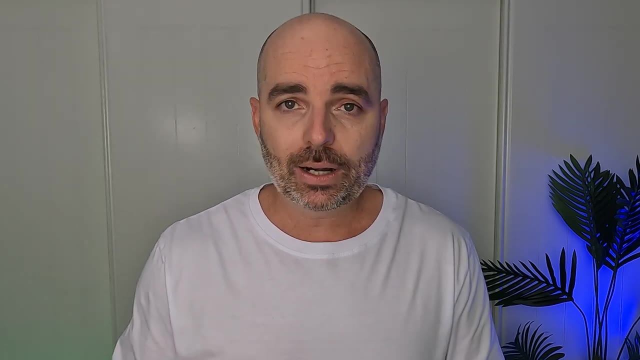 that and then start marketing those other products or services. So, going back to that example of electrician, let's just say you started with your air conditioning services And then after a couple of months, you got some more air conditioning jobs, which is bringing more money into your business. 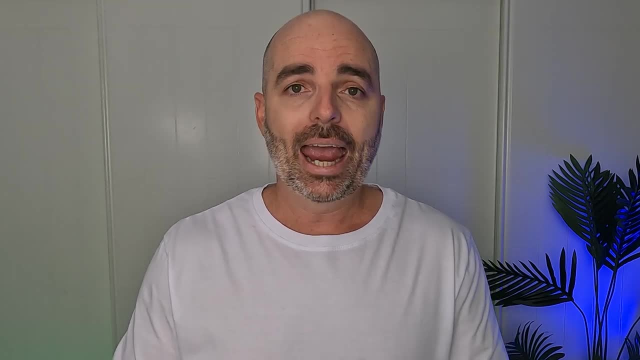 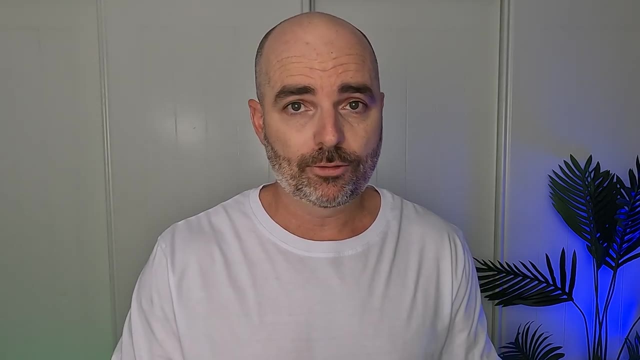 you are then able to reinvest some of that revenue and then go about and market your general electrician jobs. So with this we're going to talk about how you can start marketing those other products or services. And this strategy it's all about focusing on your strengths: first, increasing the revenue coming in so that you've 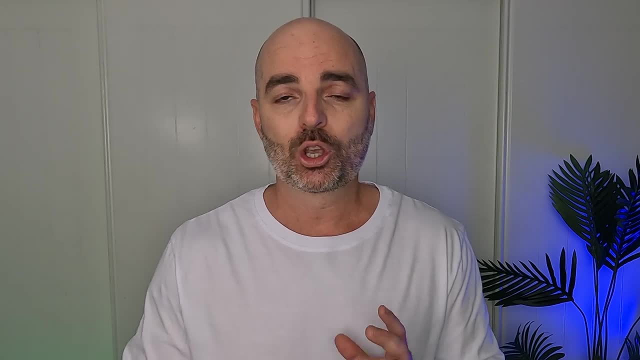 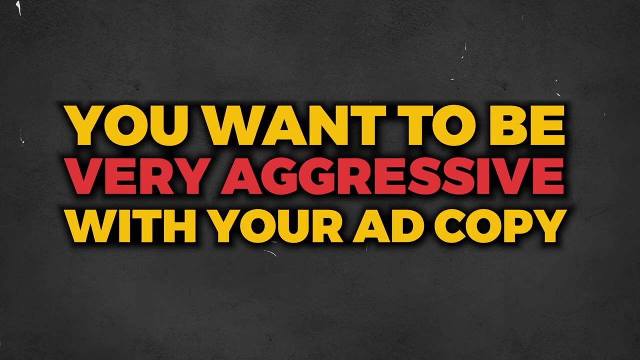 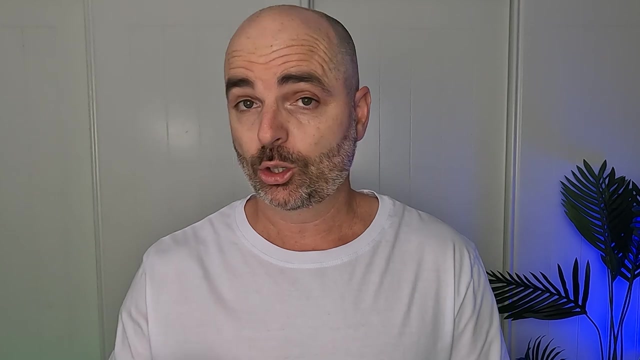 then got more money to reinvest into marketing your business with Google Ads. And then that brings us to the third and final strategy, And that is that you need to be super aggressive with your ad copy. And the reason for this is that- remember, with Google Ads is that you only pay when someone clicks on your ad. So by having super aggressive ad copy, it's better. 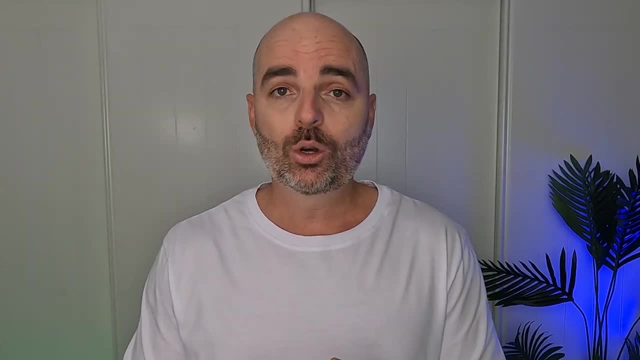 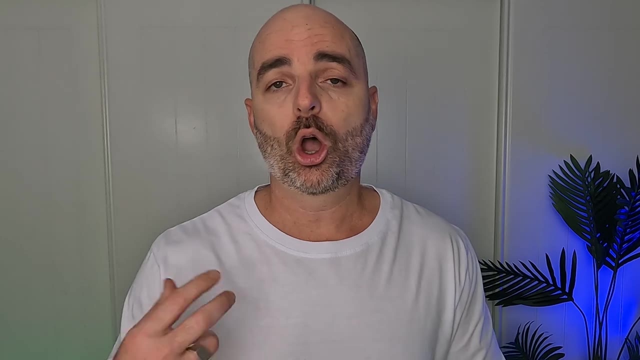 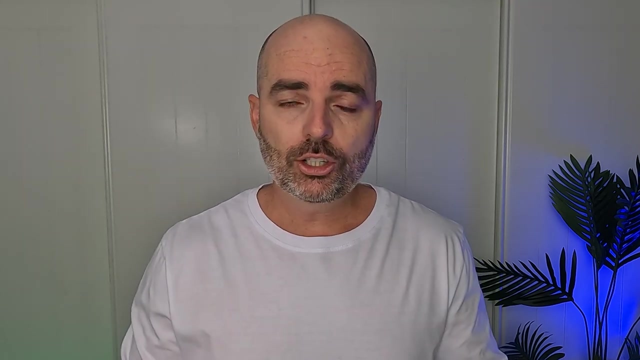 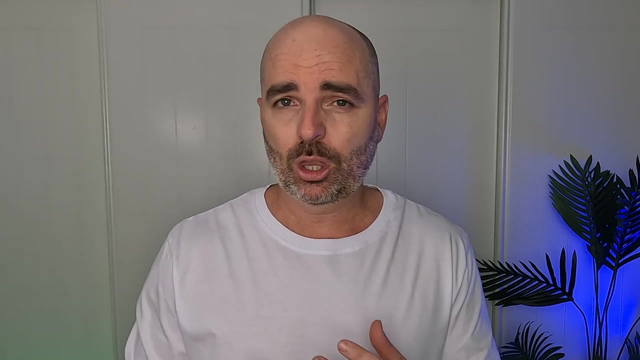 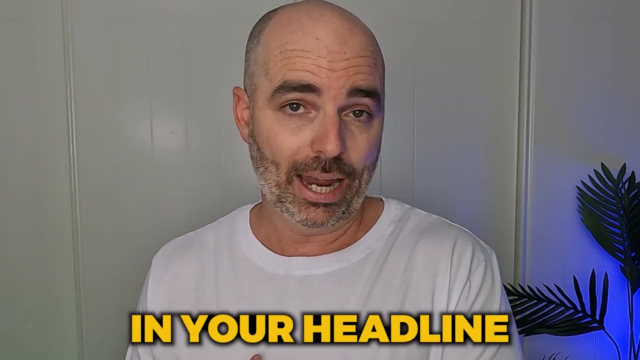 off for someone to see your ad And not click on it, because what a worst scenario would be is that, if they then see your ad, click on it- you're then charged for that click- for them to only go to your website and then bounce off in a couple of seconds because it's not exactly what they were looking for. So what you're wanting to do here is that you're wanting to put as much specific information as possible in your ad copy so that you can filter out some of those clicks which you know are just going to be a waste of time, And some great examples of this is, firstly, put a clear price in your head. 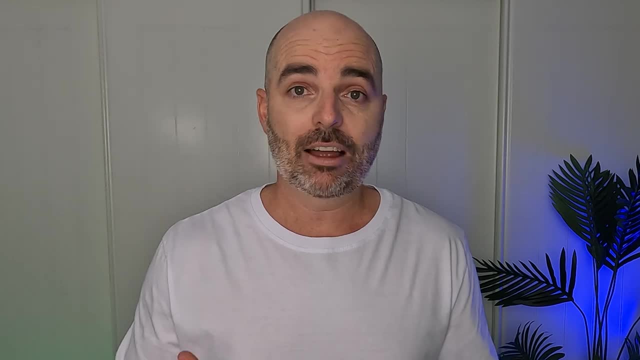 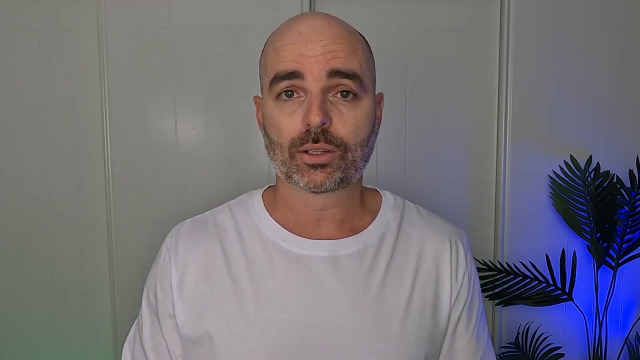 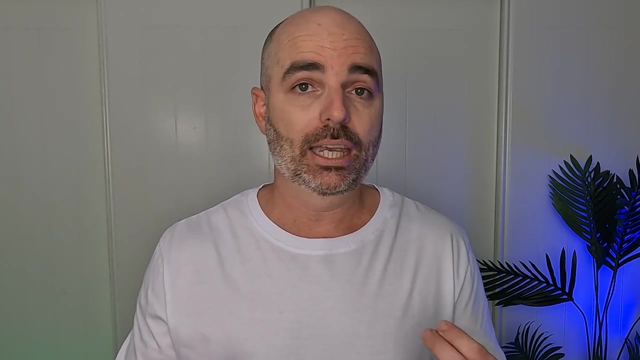 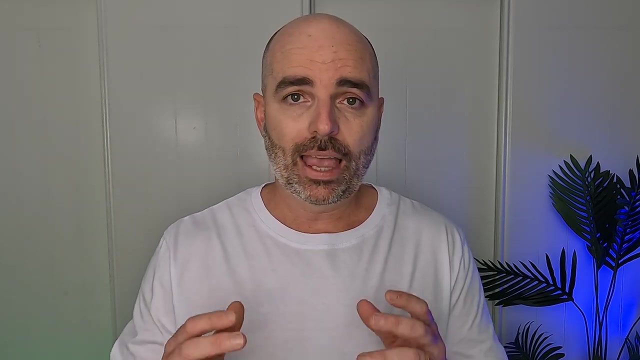 So let's just say you're running a service and your services start from $199. Now there may be some of your competitors that are willing to offer that service for $149 or $99. But by putting your price right there in the ad copy you're then going to be filtering out those people who are happy to pay $99 or $149 for a product or service which doesn't have the same level of quality. So a great way of helping to limit that spend is by putting in a clear price market in your ad copy. 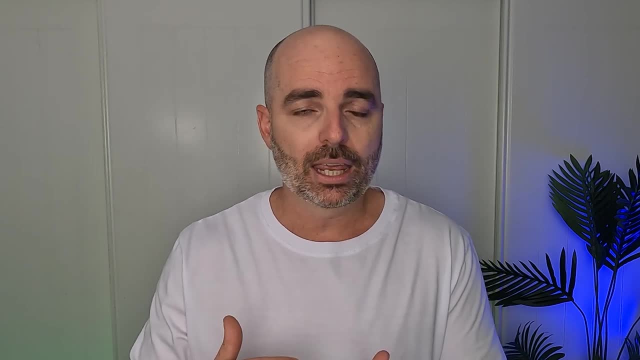 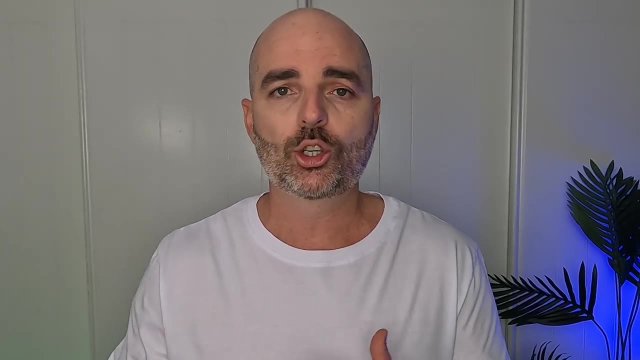 And then the second way- and this may sound counterintuitive, but to put in some clear limitations about your products, Because remembering here that what you're wanting to do is you're only wanting to get that click for people who you know are gonna have a better chance. 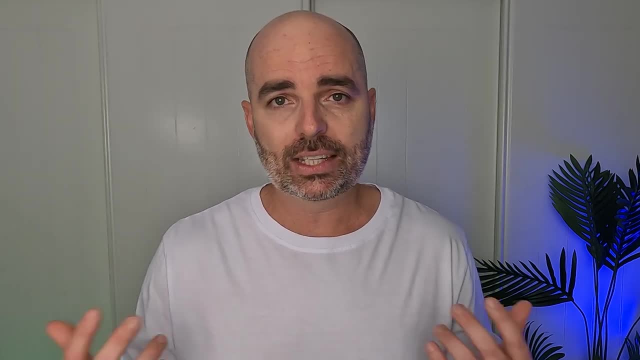 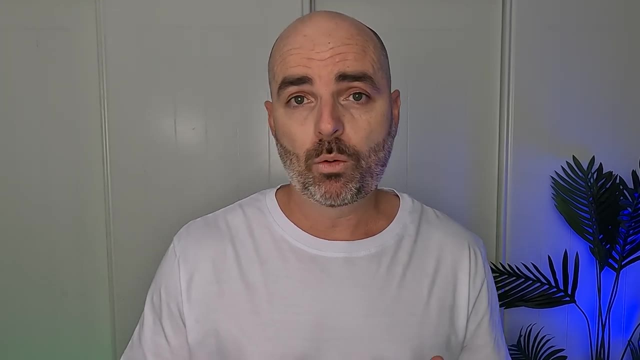 of buying your product. So an example of this is remember how I said at the start of this video that the first campaign that we ran was for our own tourism business And in that campaign we were marketing our one bedroom villas. So what we did is that we made it very, very clear. 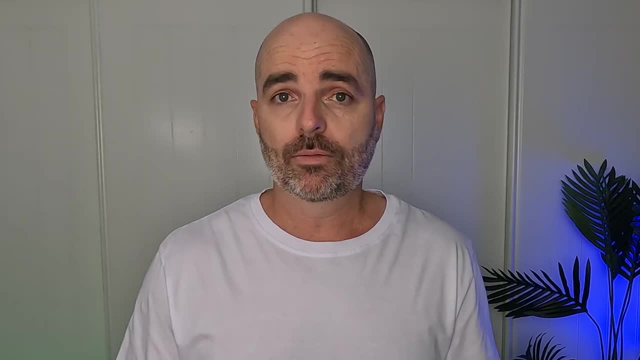 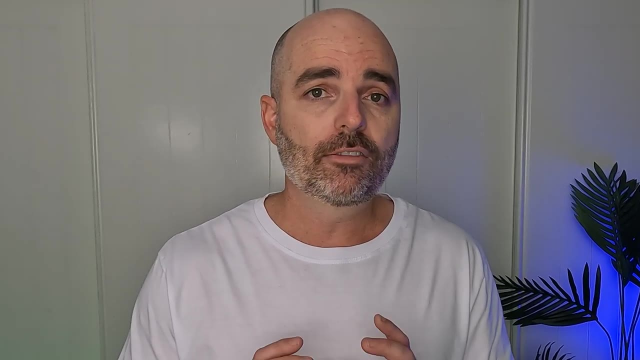 that our accommodation was only for couples, Because we had one bedroom villas that only had a king size bed in it. we didn't want to attract that family market or people traveling in groups. So we made it very, very clear that our villas were very much for couples. 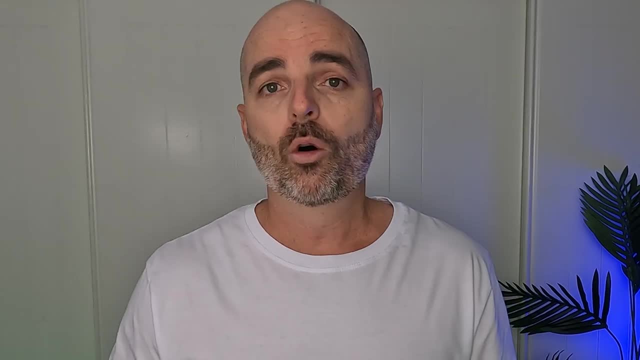 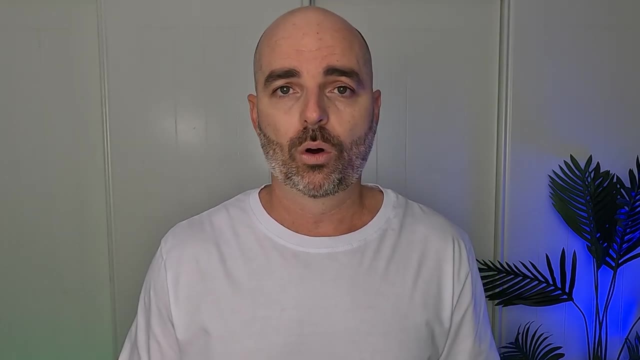 So we also added in there that they were perfect for honeymoons or perfect for couples traveling without kids, And what this did was that it stopped us getting a lot of wasted clicks for people who are wanting to look for family holidays or, as I said, people traveling in larger groups. 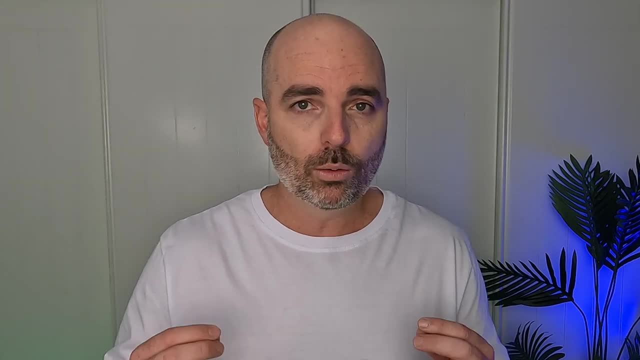 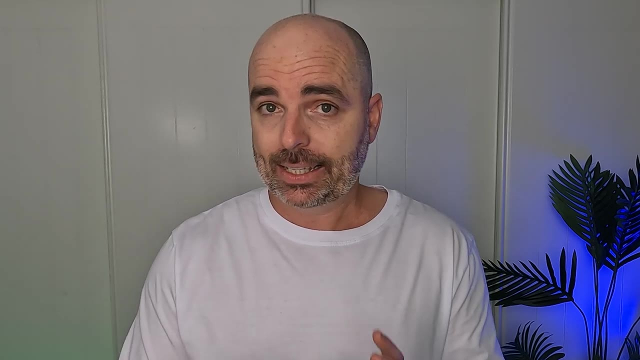 So that one may sound counter-intuitive, but I hope you understand what we were achieving there, Because for us we found it a very, very successful strategy. So if you're running Google ads and you need to see success with a small budget,